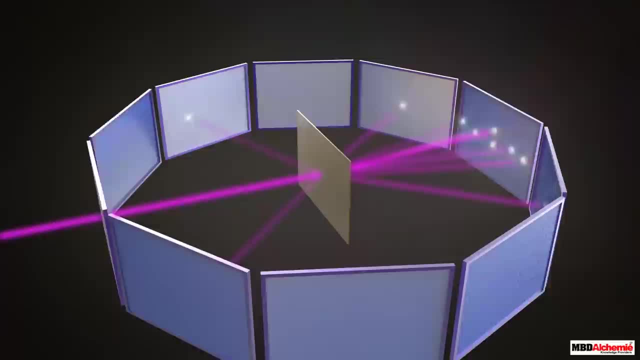 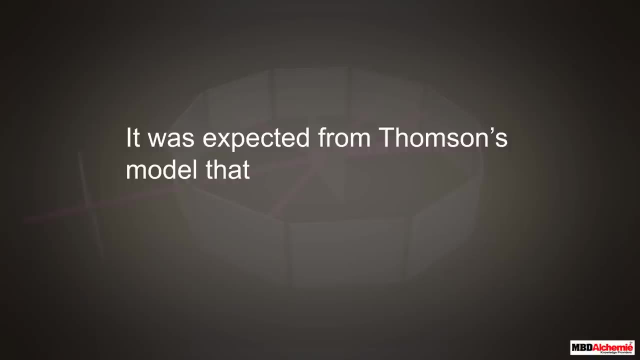 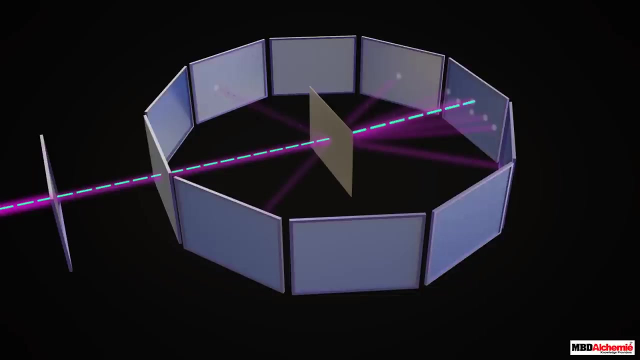 the gold foil and got scattered in different directions. their scattering pattern was shown by the detector. it was expected from the thompson model that it should show a large number of deflections, but something else was observed. actually, the detector showed that most of the alpha particles passed through the gold foil as such, without 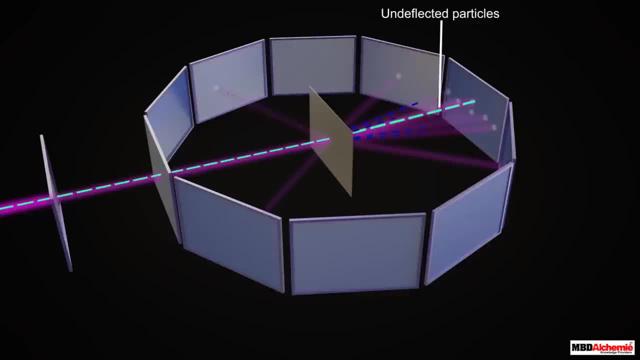 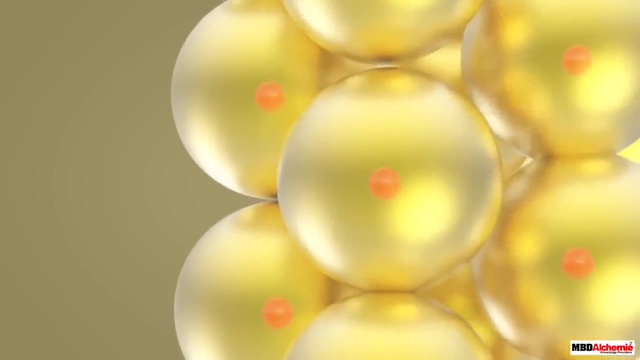 showing any deflection. only a few of them showed deflection in different directions. a very few of them, essentially one in twelve thousand, rebounded back. such observations led to significant conclusions. let us see what those were, as most of the particles passed through the gold foil during the time of the deflection z. 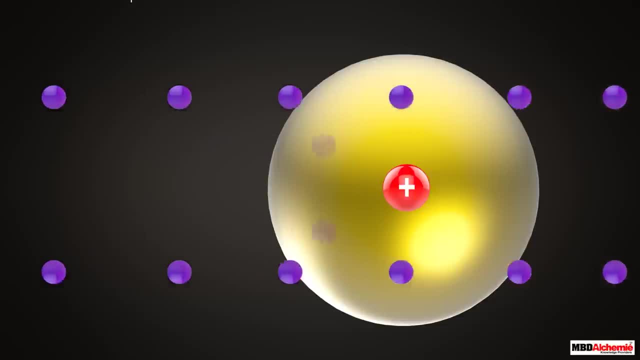 undeflected. Rutherford concluded that most of the space inside a gold atom was empty. A few particles were deflected from their path by small angles, indicating that there must be a positively charged center which was repelling alpha particles. As these particles 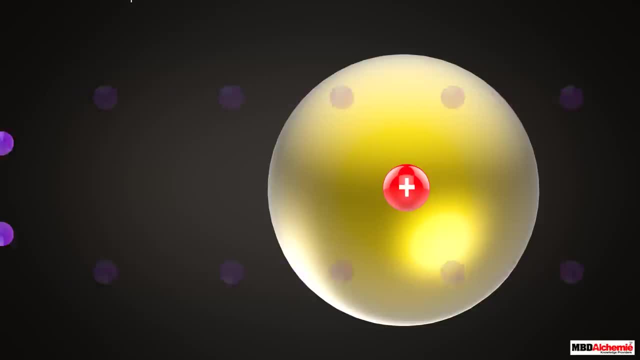 were few in number. this led to the conclusion that a positively charged center occupies a tiny space. The few particles that are rebounded back indicate that all the positive charge of the atom was concentrated in a very small volume in the center Rutherford named this. 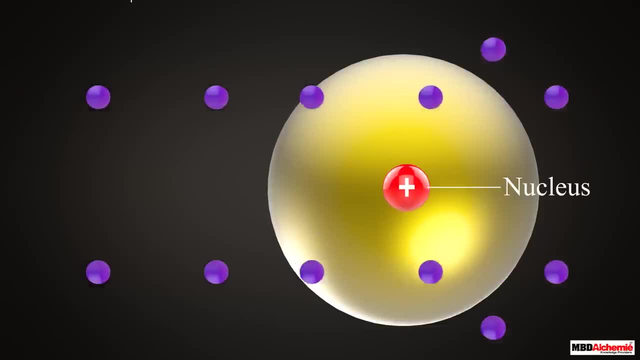 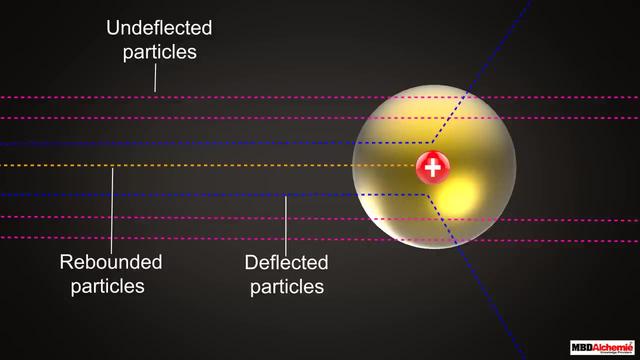 positive center of the atom as a nucleus. Looking at the proportion of the particles undeflected, deflected and rebounded, and based upon some calculations, Rutherford concluded that most of the mass of an atom is concentrated in its nucleus. Subtitles by the Amaraorg community. 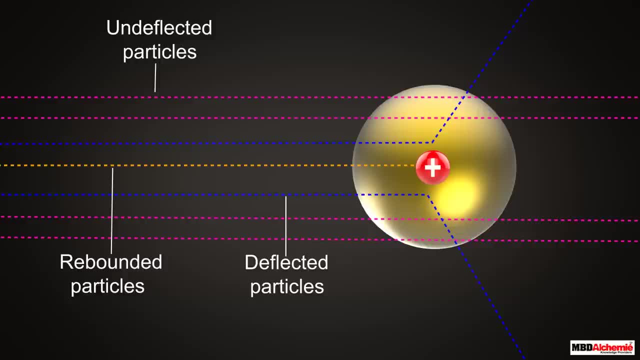 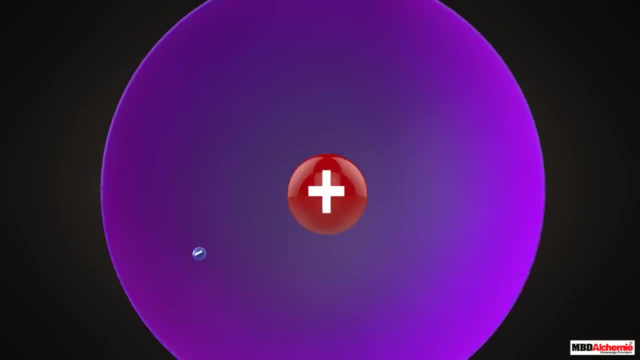 Based on all these conclusions, Rutherford suggested an atomic model, which was known as the nuclear model of atom. According to Rutherford's nuclear model, there is a positively charged center in an atom called nucleus, and all the mass of the atom is due to this. 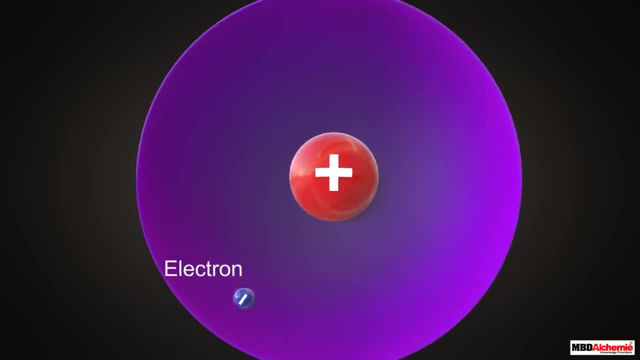 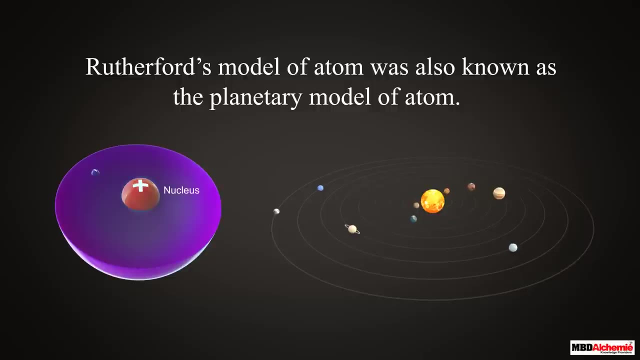 nucleus. It also suggested that electrons of the atom revolve around its nucleus. This model is called the nuclear model of atom. The nuclear model was also known as planetary model, as the nucleus of the atom can be compared to a miniature sun and electrons revolving around the nucleus can be compared to the.